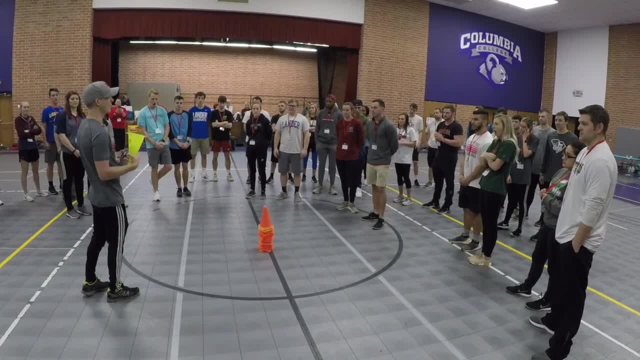 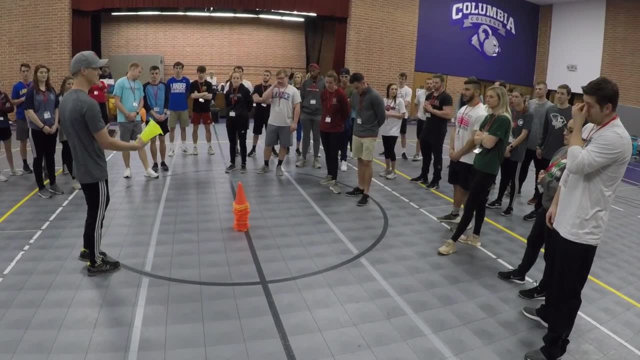 great warm-up activity. This is also a relay we do on field day and a great way to work on good sportsmanship and learning how to win and lose. So learning how to be a winner that wins in a good way and has good sportsmanship, and also learning how to lose a game Okay. so, for example, can you? 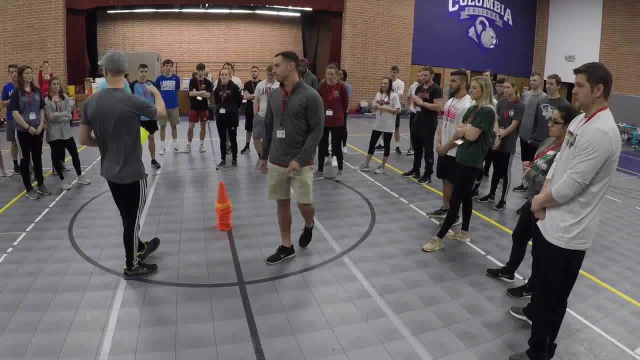 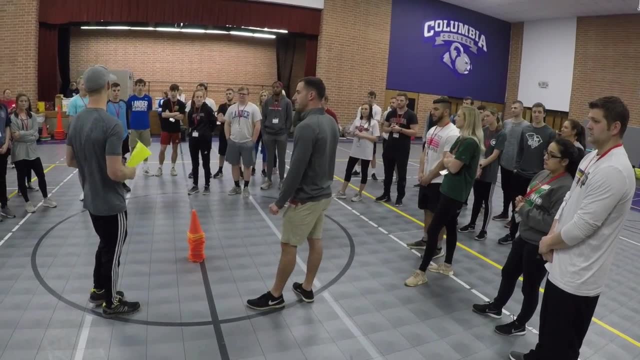 help me do a quick demo. Okay, we're going to just stay inside this yellow square area. What you're going to do is you're going to practice cone flipping. Why cone flipping? Because kids love to do it. Like three years ago, the bottle flip thing was so big, so they just love to do. 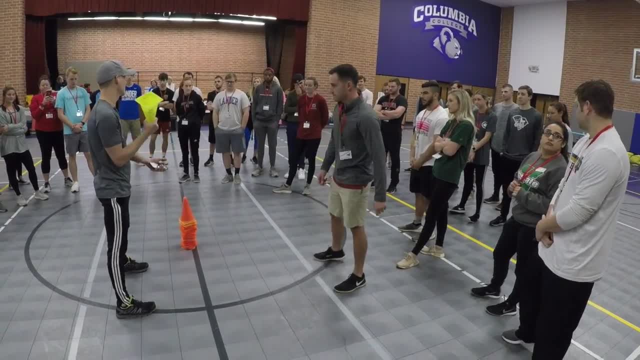 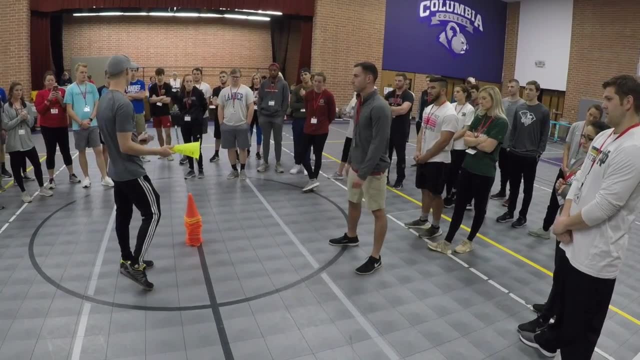 the cone flipping And it's just an easy way for you to, instead of doing something like rock paper scissors. you can do the same thing with rock paper scissors, but the kids really love doing the cone flip, So you're going to just take turns, going back and forth, First person to flip. 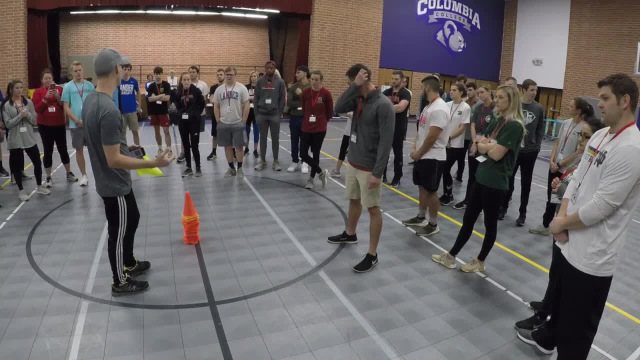 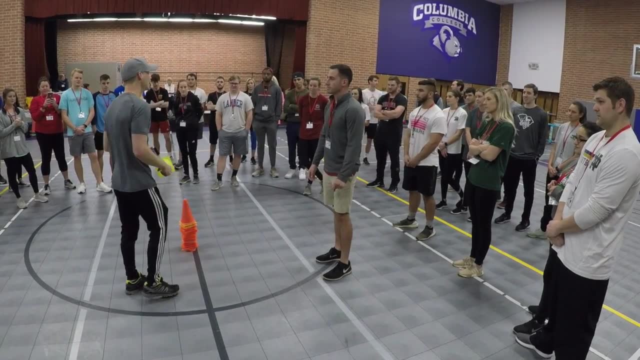 the cone and get it to land up is the winner. When you win or when you lose, you're going to do a handshake, a fist bump or a high five and say good game. Everybody say good game. Winner's going to stay, raise their hand. Loser's going to jog one time around, get back in the game and 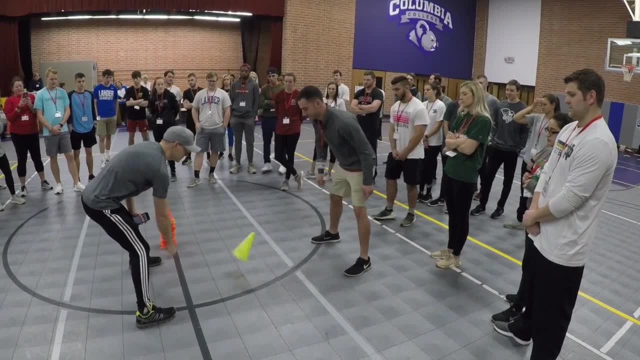 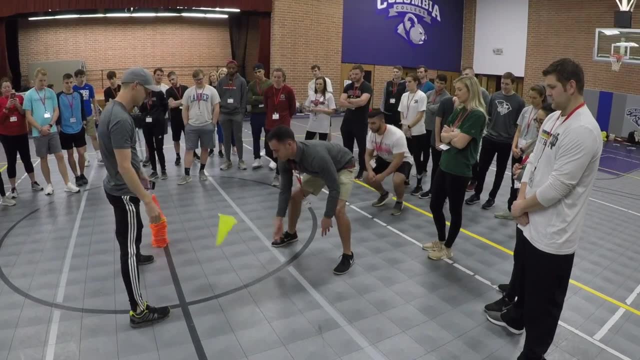 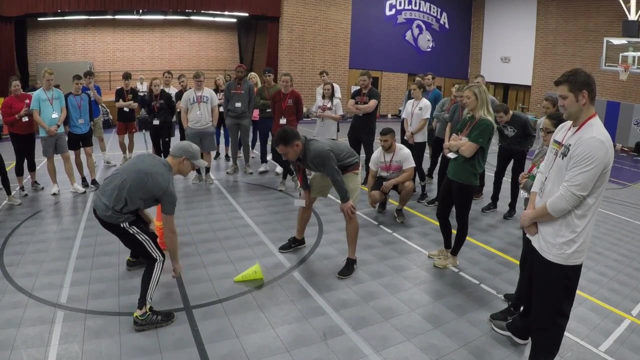 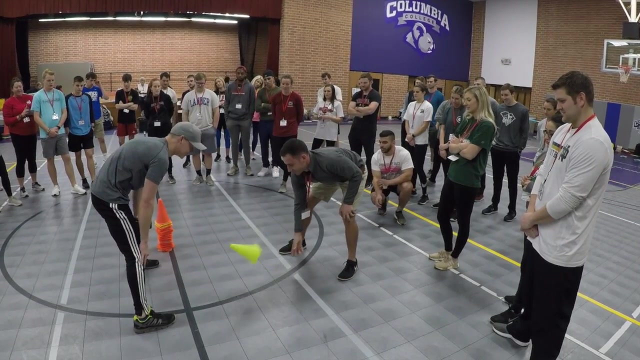 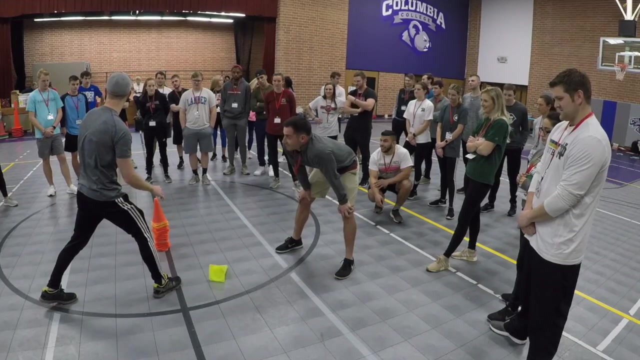 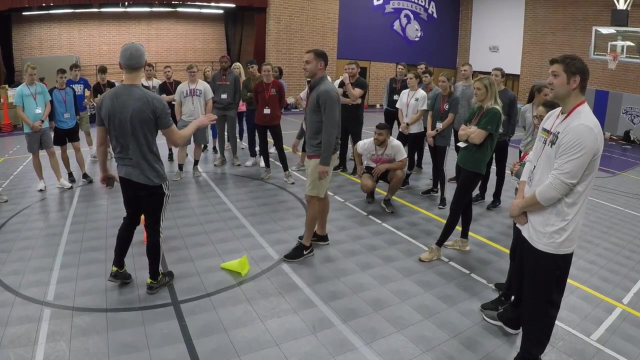 find a new partner to play. Okay, you ready, Might be here for a while. Oh, so close. This floor is pretty rough. We might need to modify this game in a minute. All right, due to the nature of this floor, we're going to say after 10 flips. 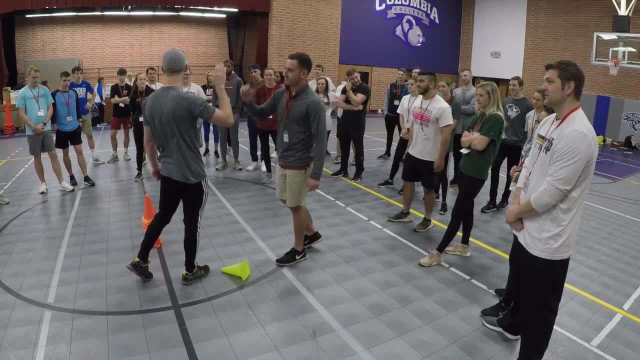 10 flips is a tie. Handshake, fist bump or high five Say what Good game. If it's a tie, you can both jog a lap together, but then come find a different partner in the middle. So you're. 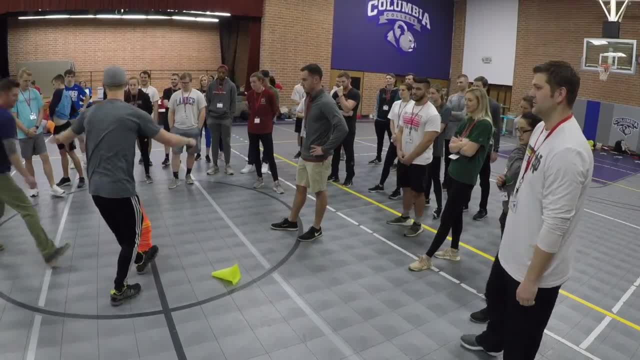 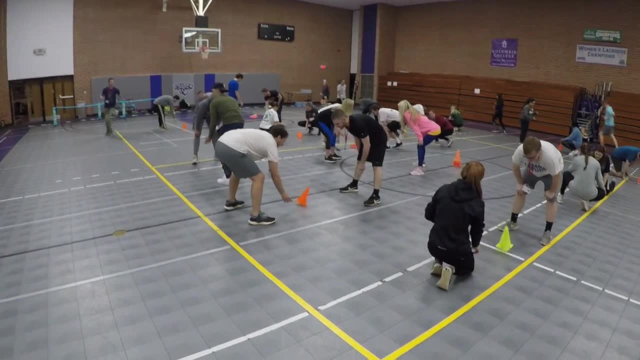 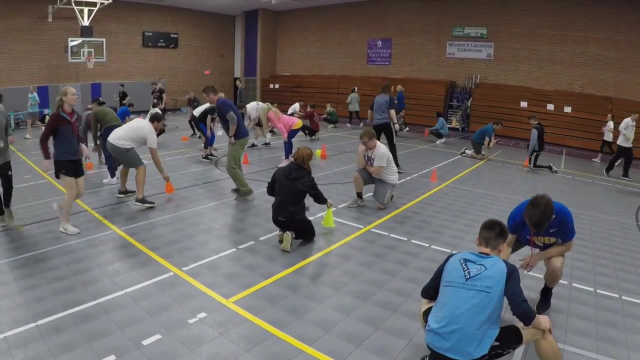 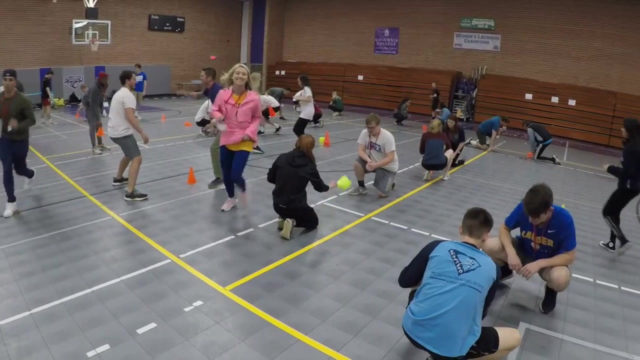 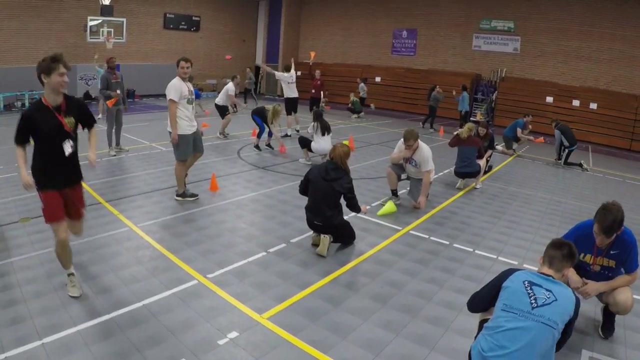 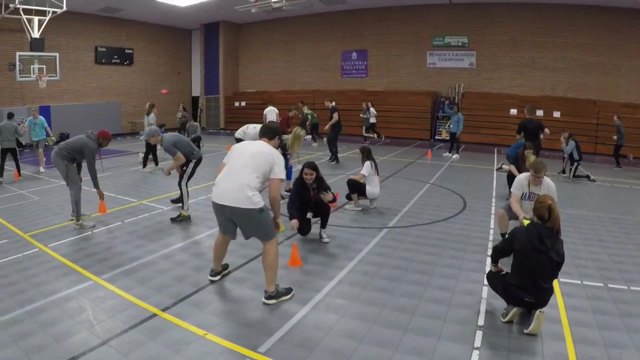 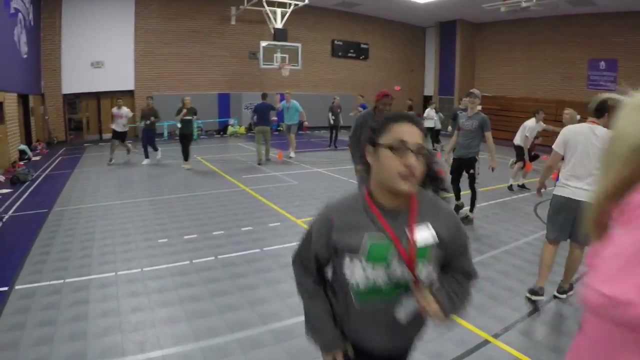 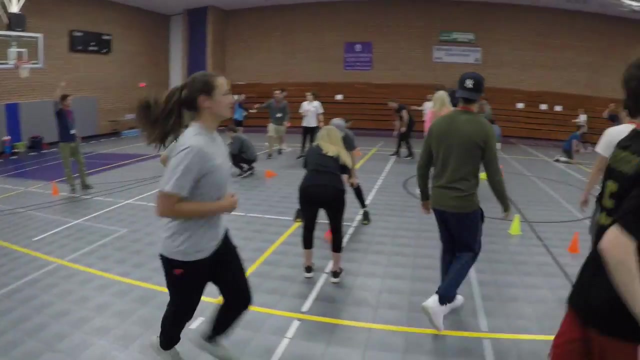 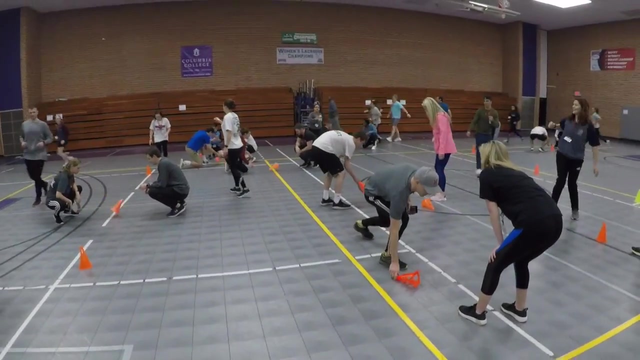 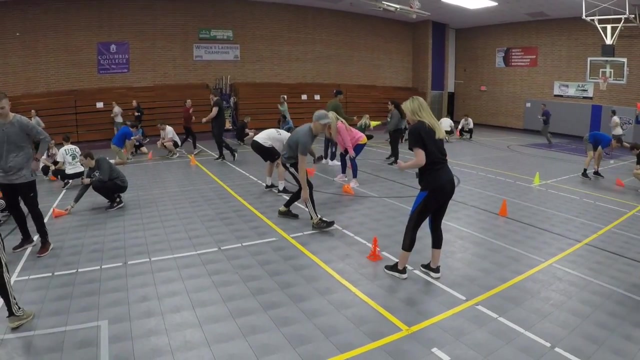 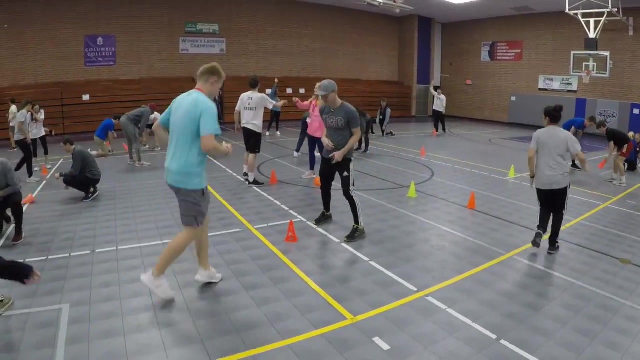 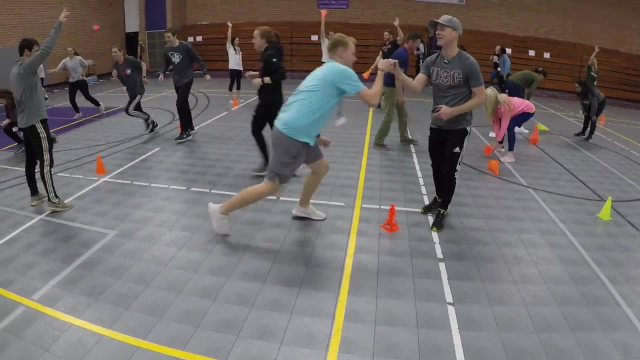 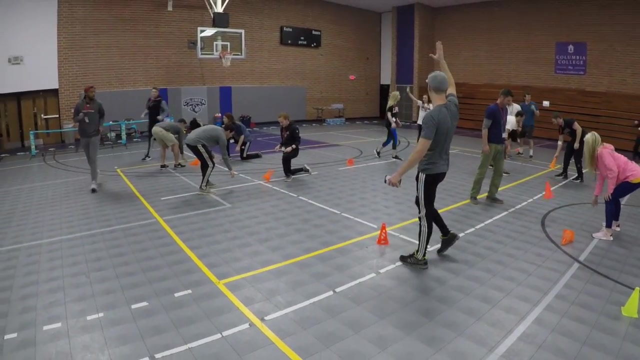 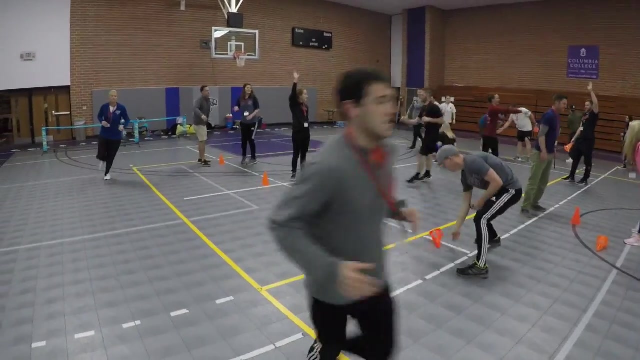 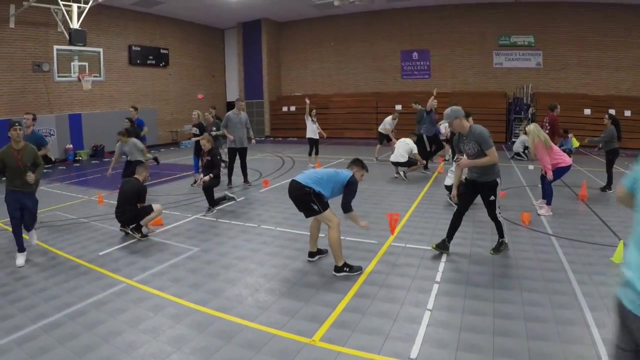 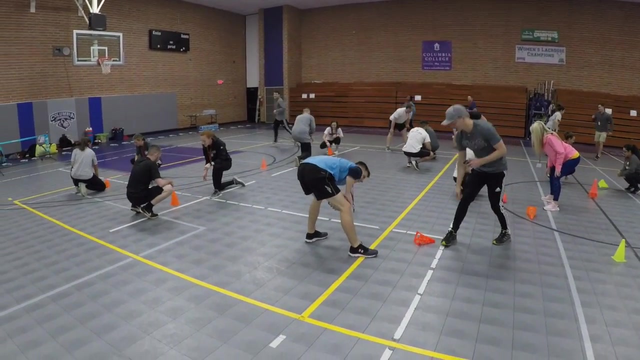 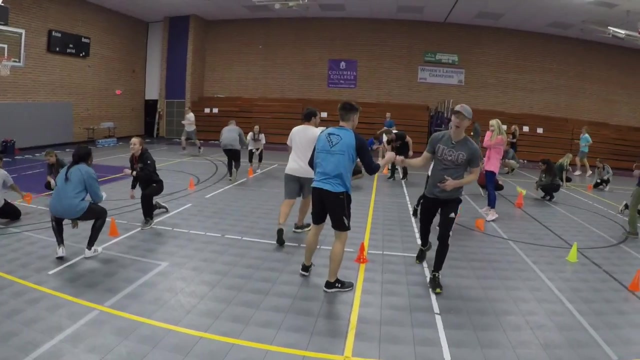 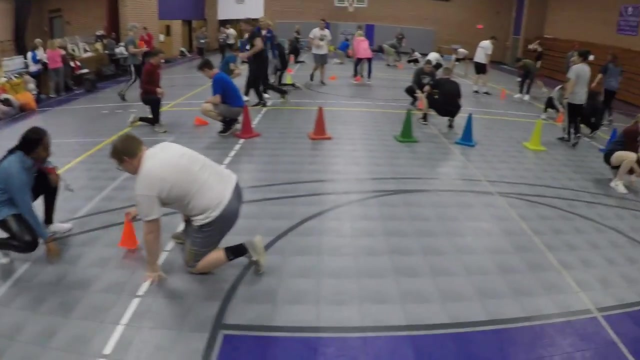 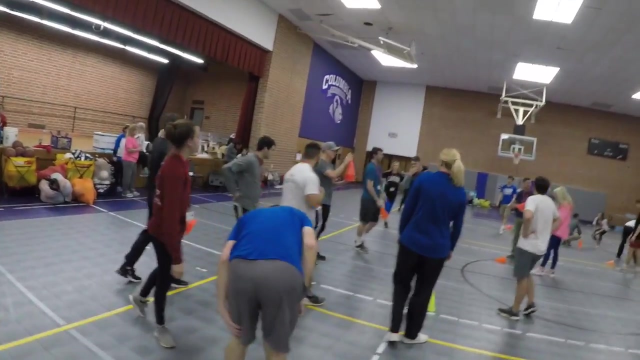 switching up your partners Make sense. Come grab a cone, Spread out in this white square, white square, Oh yeah, Oh, Oh, Oh. All right, referees, Okay, bring the comb. and then I need groups of six behind these six cones, right here, groups of six. 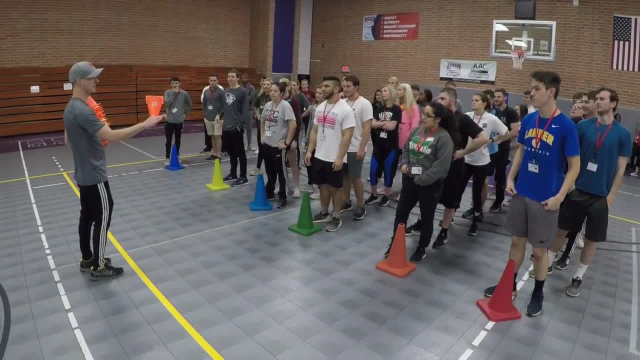 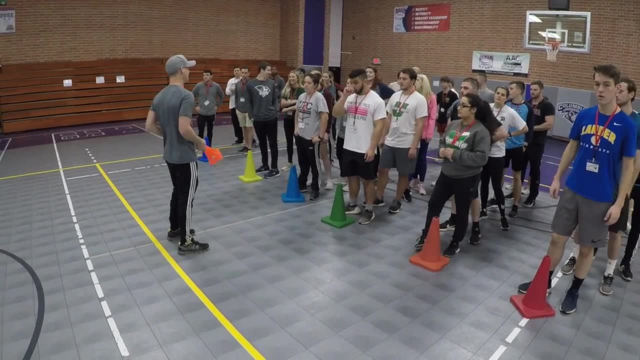 All right. so Not appropriate for PE to have lines of six. This is a Relay style thing that we do for field day. So we Do that cone flip game in PE. everybody's moving and we do a relay style game for field day. The kids are rotating around to different stations all in four different teams. 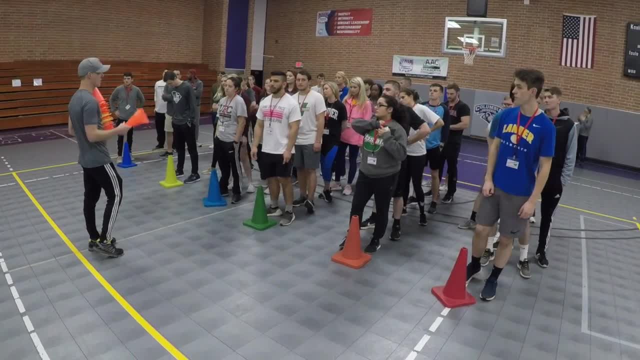 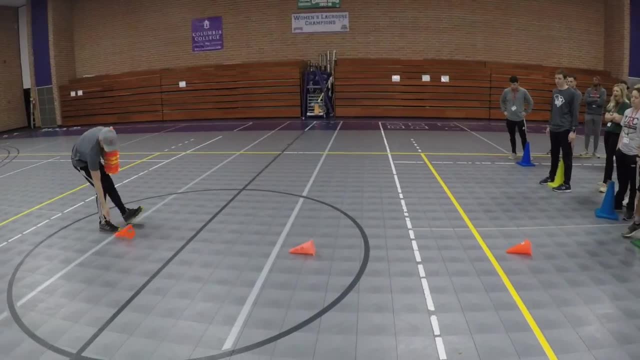 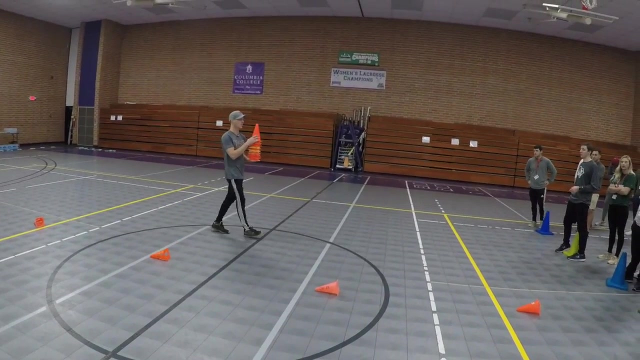 So if you have more equipment you could make as many lines as you want. first person lines gonna help me out. They're gonna come and lay the cones down in a line and We'll go with One, two, three, four, five. Okay, so for these small cones, first person, just lay them down in the line. 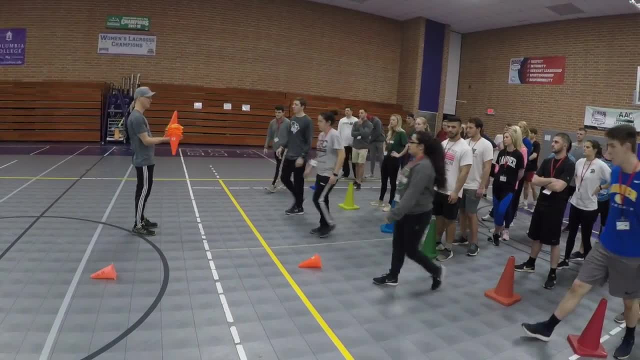 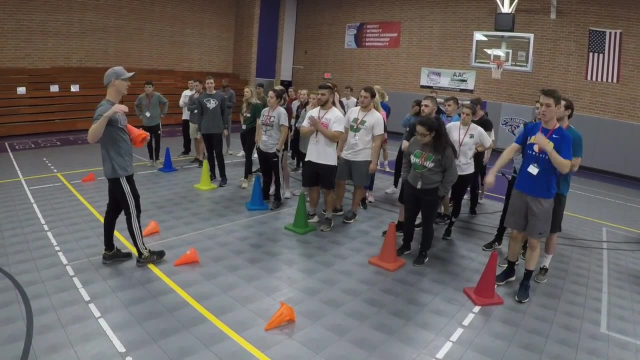 The big cone will be the last one. All right, go, Thanks. so the way it works, first person's gonna run down. you get one flip. How many flips do you get one flip as fast as you can run back? tag next person. You cannot leave the call until they tag your hand once you flip it up. 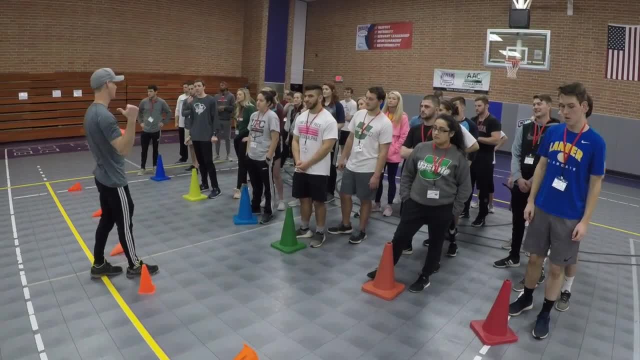 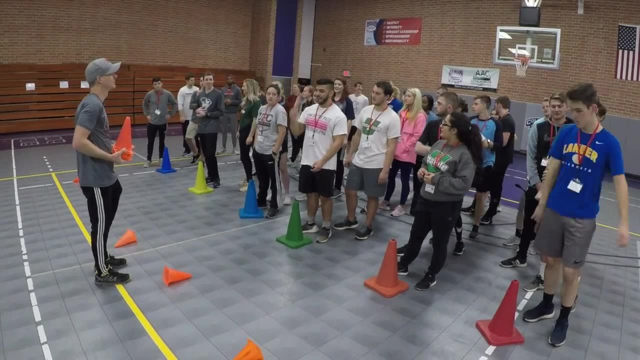 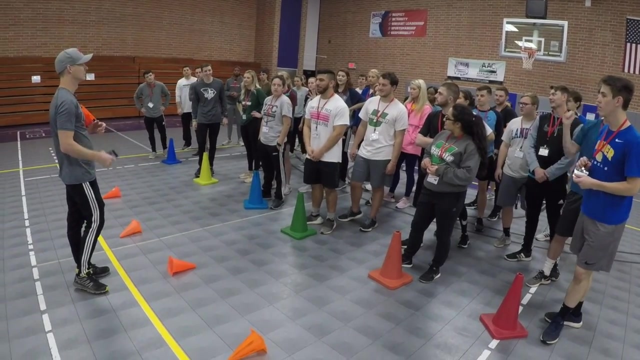 Next person you leave it up is gonna run to the next cone and flip it first. seem to flip their big cone Will be the winner of the cone flip relay. Yeah, Oh, sorry, I bet. Great question. So if you can't flip the cone, how many flips you get one? So let's do a quick demo. 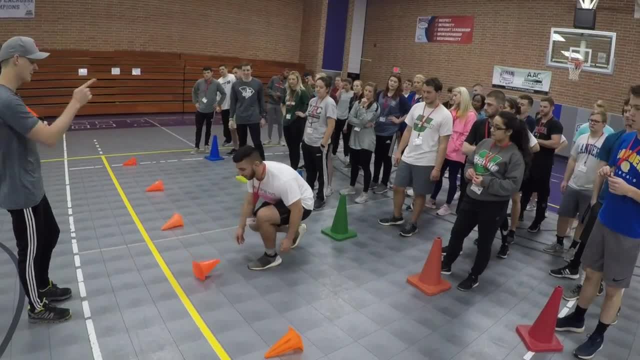 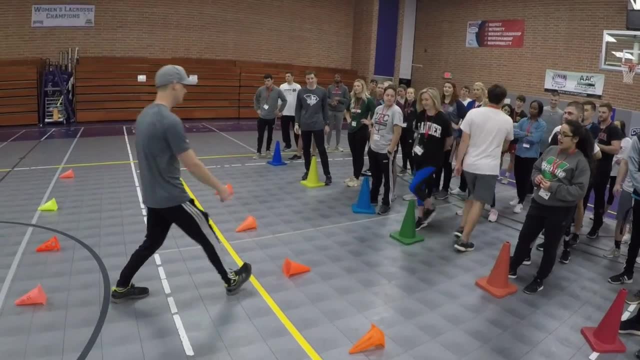 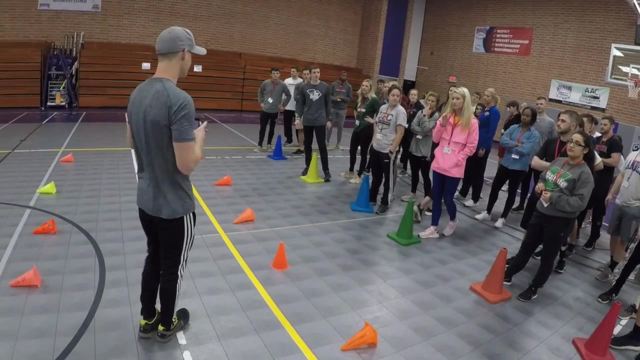 So come down and do the flip Run back, tag next person, Go the back line. come up, flip, tag next person. if she lands it, She still only gets one flip, but she'll tag next person and then you will go to the second cone. make sense, All right. 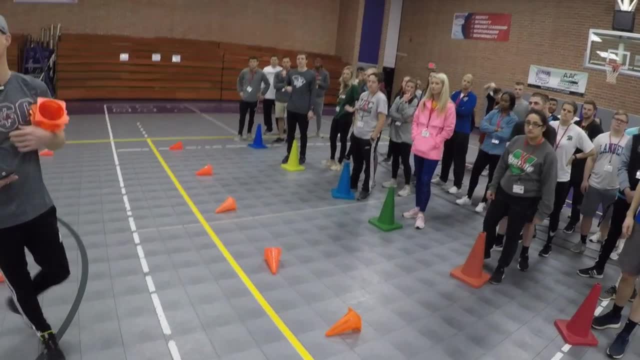 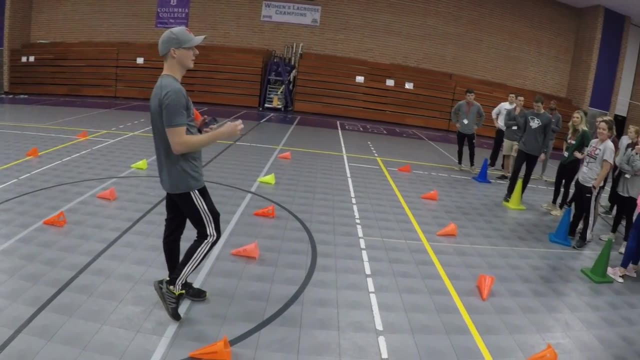 You land it, you don't go to the next, you go to the back of the line. Yeah, Okay, You can do it either way. if you want to do like, land all five, I guarantee you, if you wanted to let them come, progress if they keep winning, you could, but I like to just make them go. 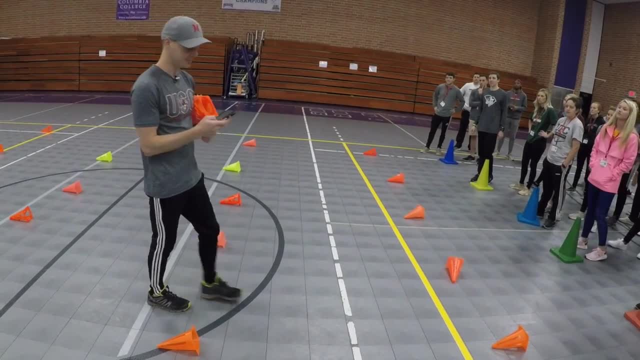 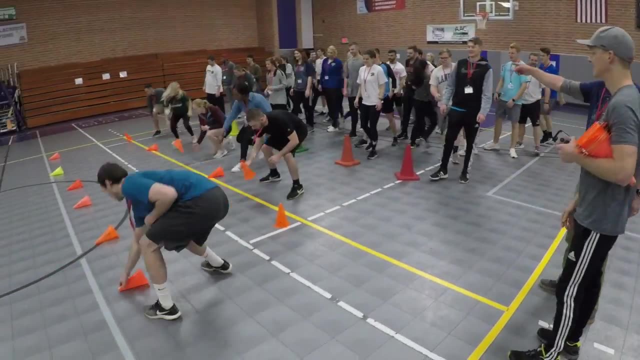 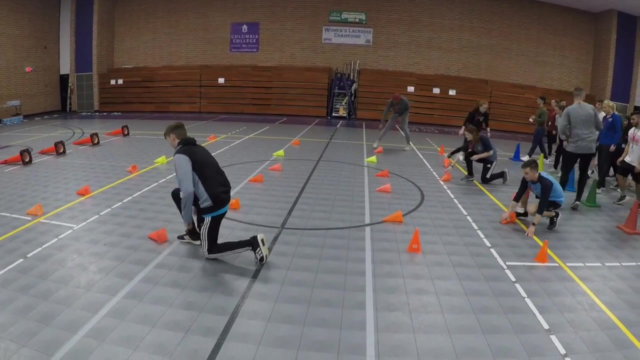 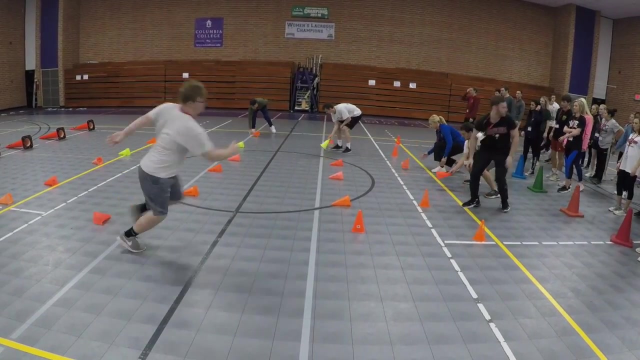 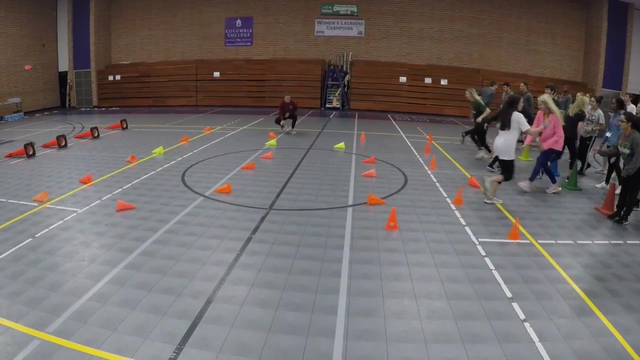 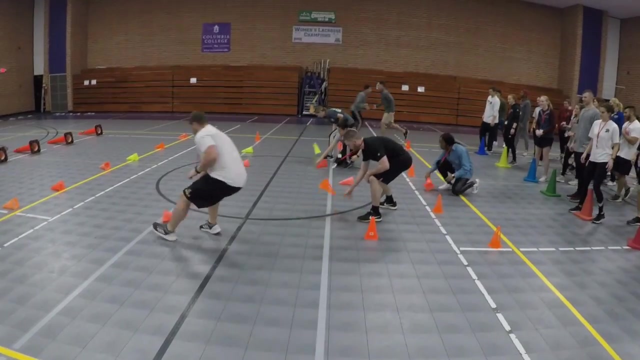 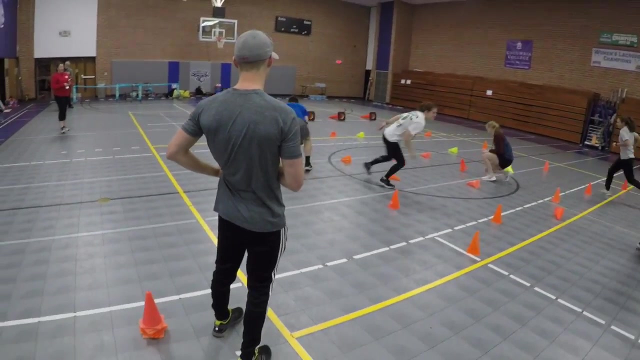 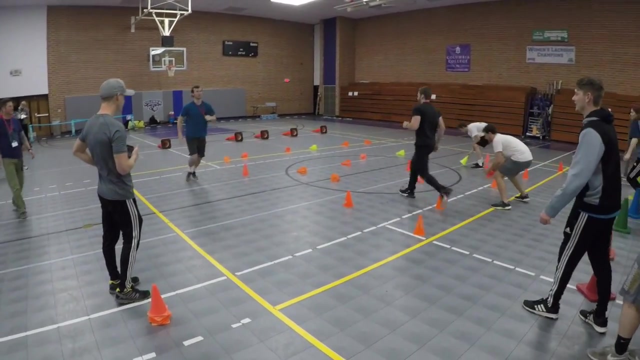 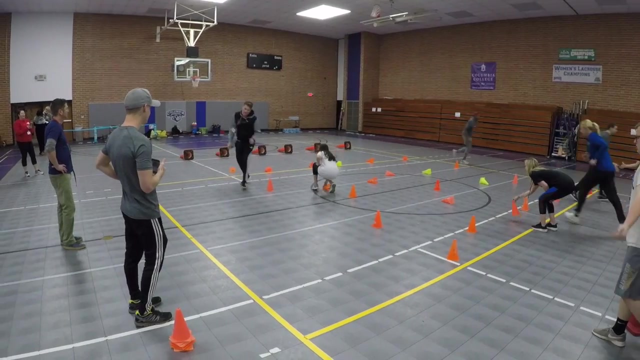 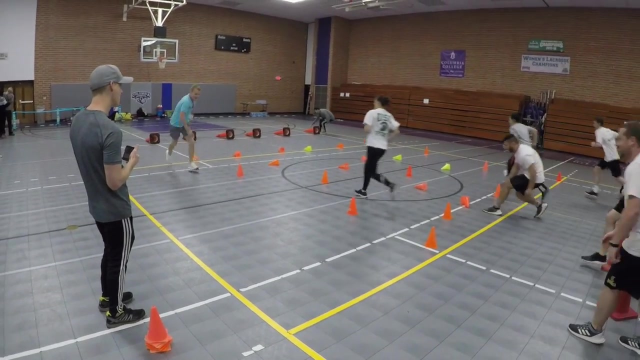 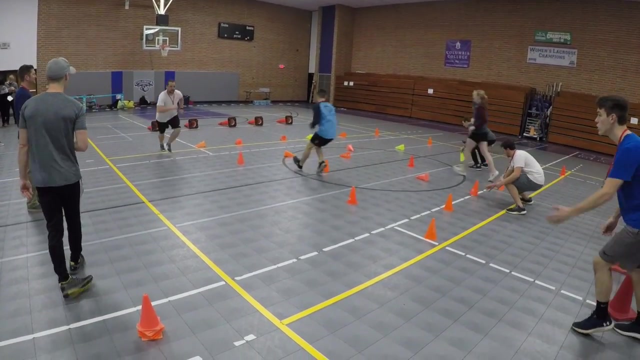